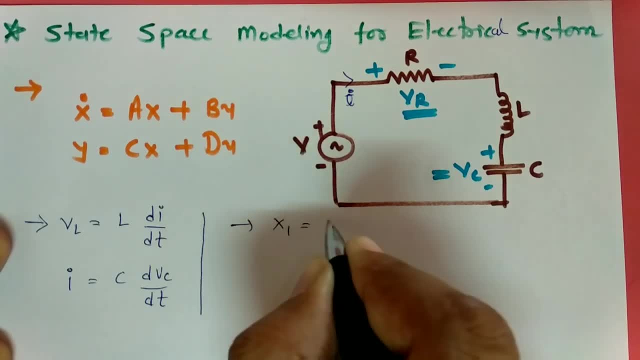 So I am considering right now two straight space variables: One is X1 and that is Vc, and second straight space variable that I am considering as current I. So second state space variable that I am considering as an I and as earlier I have told there: 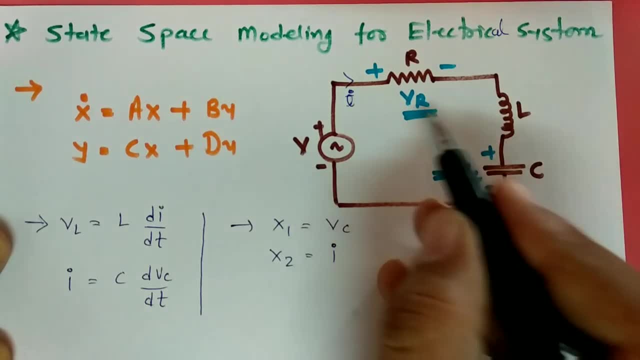 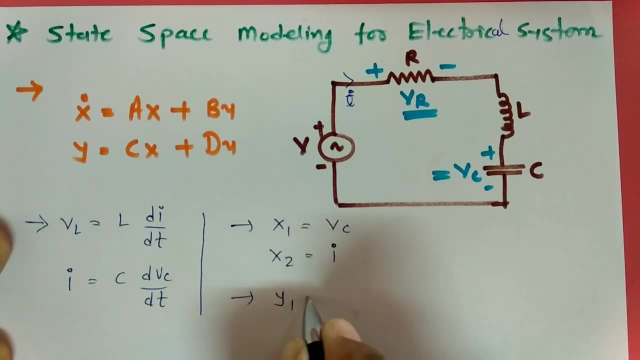 are two outputs. One output is Vr and second output is Vc. So I have two outputs in this straight space matrix: e, I1, that is Vc, and I'm considering eI2, that is Vr, and vr, that is actually i into r, i is x2. so one can say: this is what r into x2 and vc, that is x1. 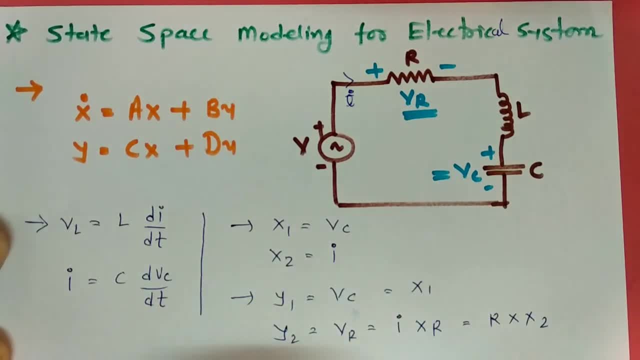 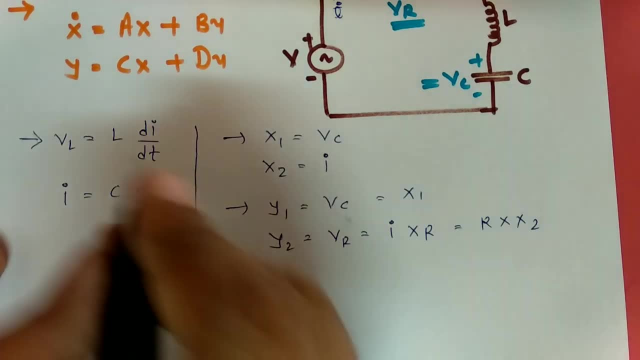 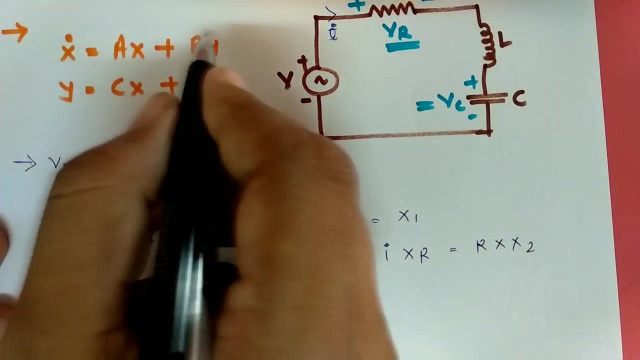 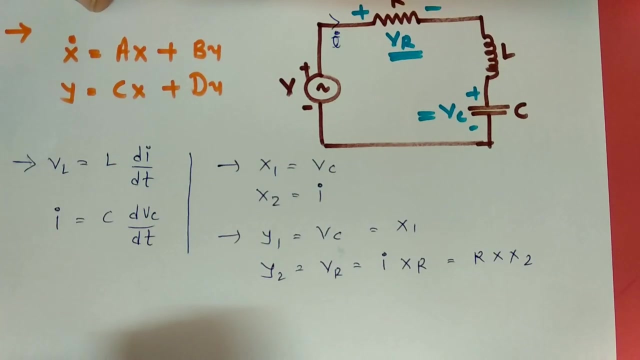 so one can say: this is what x1.. Now first I will be going to explain matrix of that x bar equation and then I will be going to derive matrix for this y. So to have derivation of this first x bar matrix, first I need to have equation for this complete loop. So for that by I will be applying. 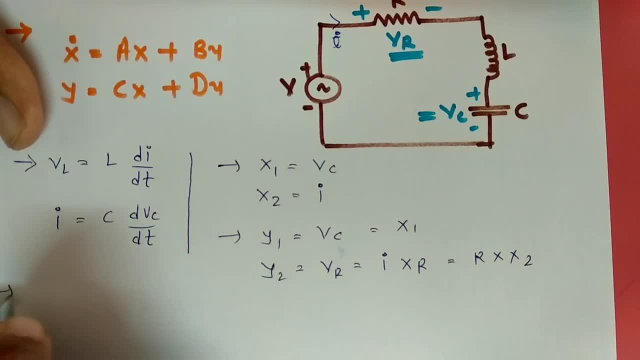 kvl, Kirchhoff voltage law. So by kvl I can be able to identify voltage v that is equals to voltage across resistance plus voltage across inductance plus voltage across capacitance. and this v, that is vr, is i into r plus vl, that is l di by dt plus vc. I am just writing vc right now. 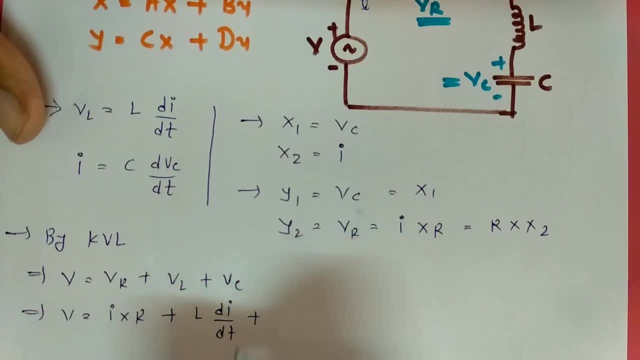 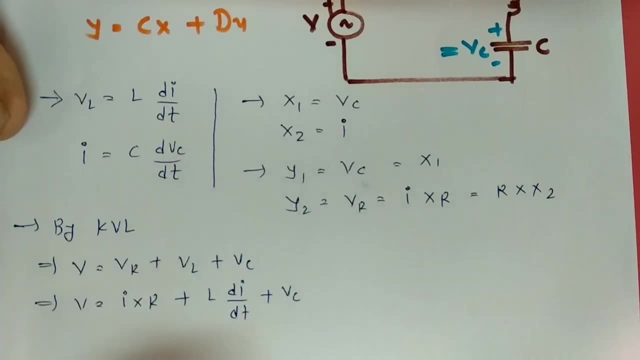 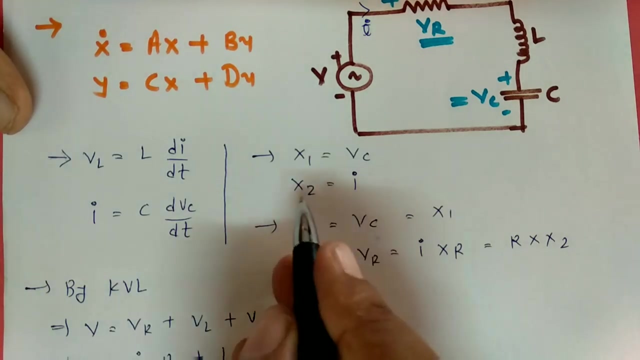 actually vc is 1 by c integration idt. vc is 1 by c integration idt, but already I have considered vc as x1, so I will be writing it as a vc. vc only over here Now, as I want to derive this in terms of x bar form. i is actually x2 and here. 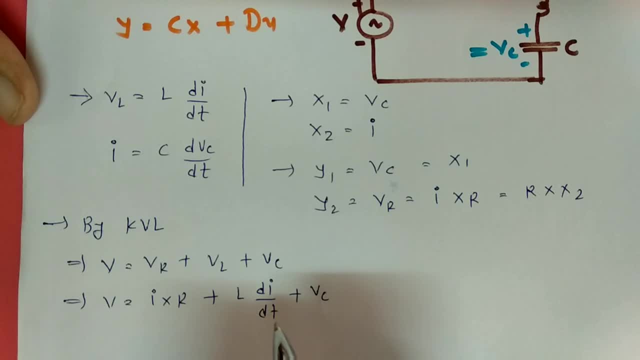 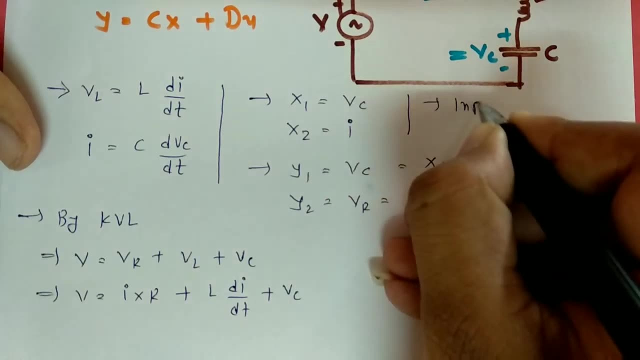 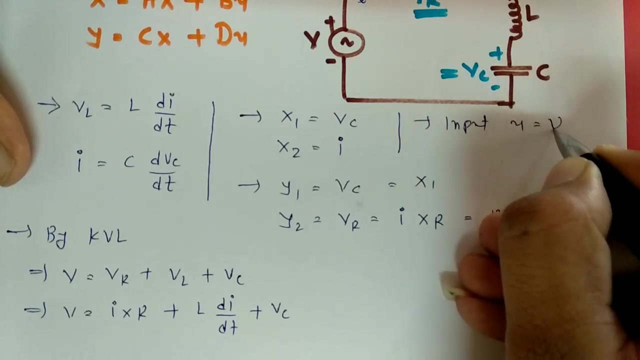 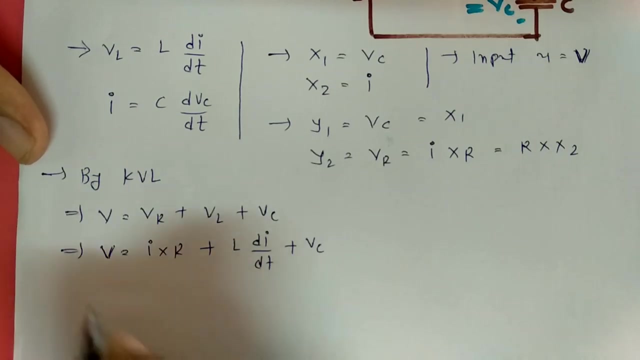 di by dt, that is x2 bar. So- and I am considering input, So input for this state space will be v. So u is equals to voltage. This is what we are applying. So here this voltage is input. So now let us place all those things in terms of state space. 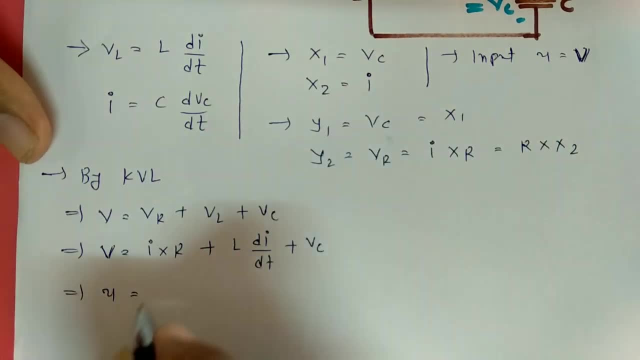 So u is equals to i, that is x2. into r plus l, into di, by dt, that is x2 bar plus vc, that is x1.. So let us rewrite this equation in terms of x2 bar. So x2 bar, that will be equals to. 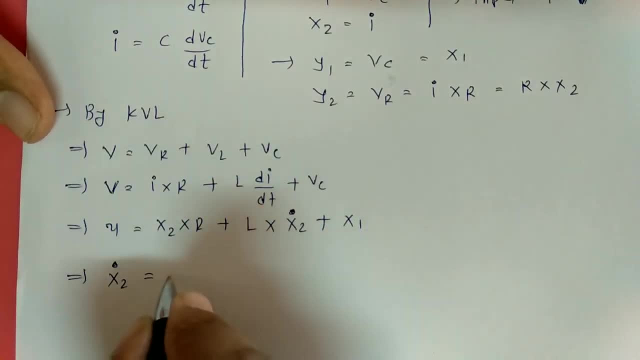 x1 will go in other side, So minus and l will be divided by entire equation to have x2 bar equation. So 1 by l into x1 plus, and even this will go on other side, So it will be again minus. So minus r by l into x2 and l is divided by u. 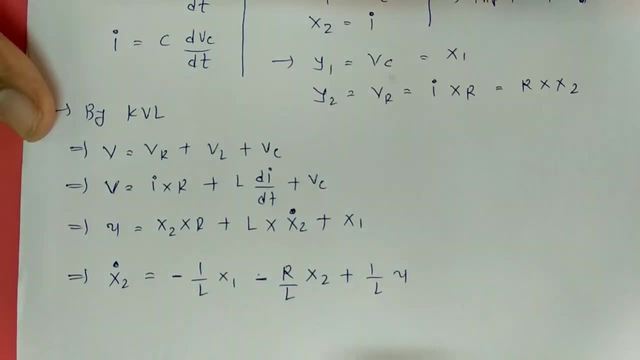 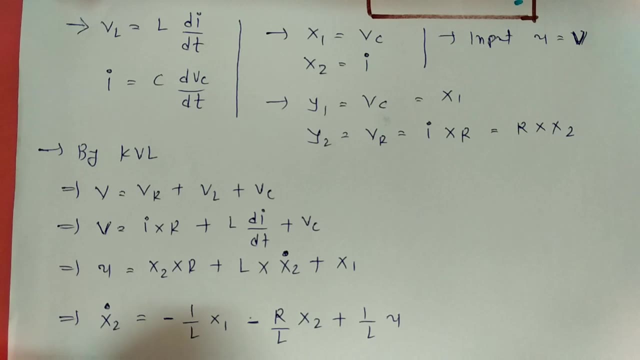 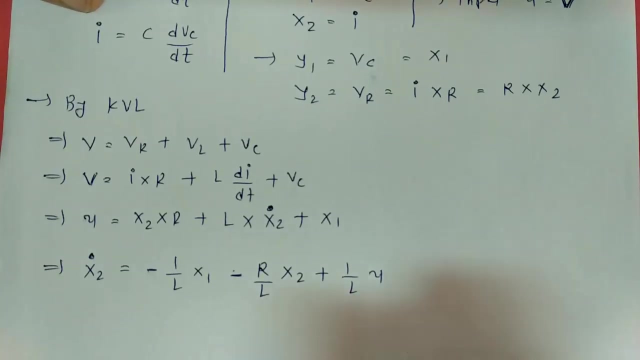 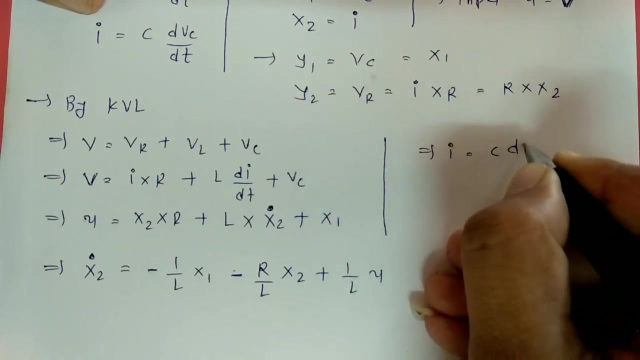 So that will be plus 1 by l into u. So this is what one equation, which is what I am having right now. Now second equation that that is this: So second equation that we can identify by i is equals to c dvc by dt. So here we have second equation, that is, i is equals to c dvc by dt, where vc that we 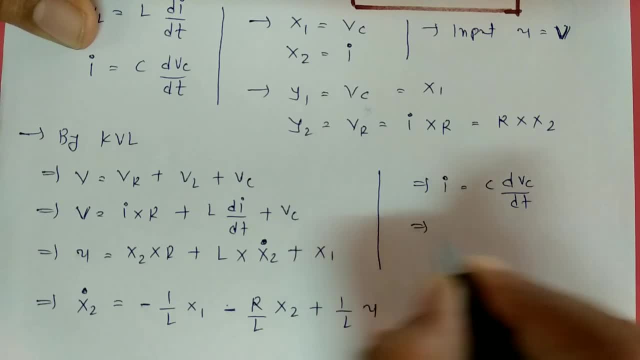 have considered as x1. So i is as x2. So i is equals to x2 and this is what cx1 bar. So our equation for x1 bar that will be 0 into x1 plus 1 by c into x2 plus 0 into u. 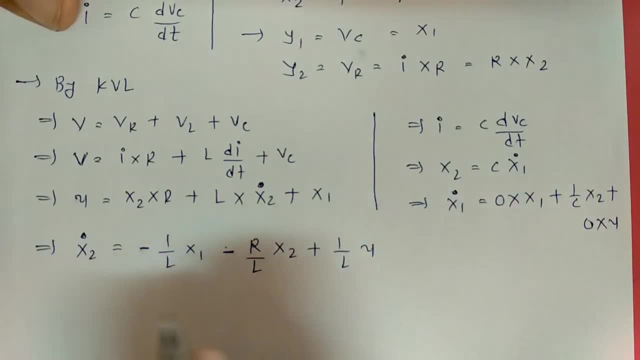 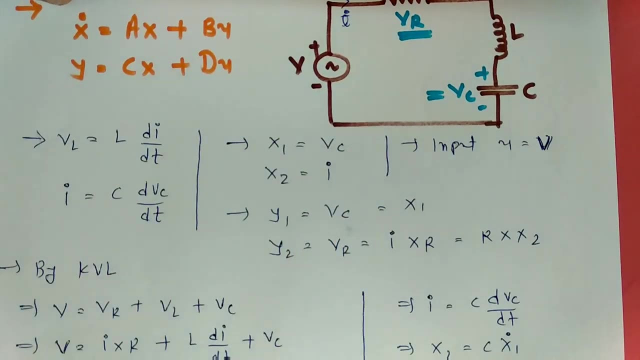 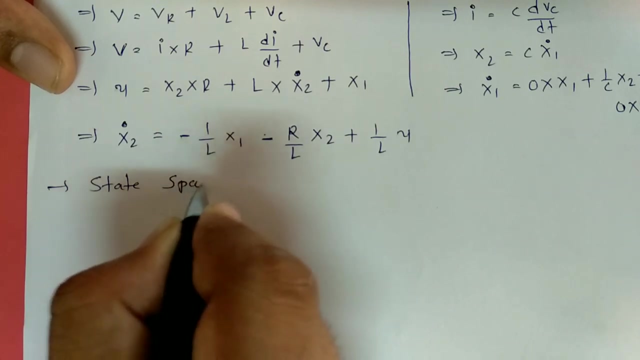 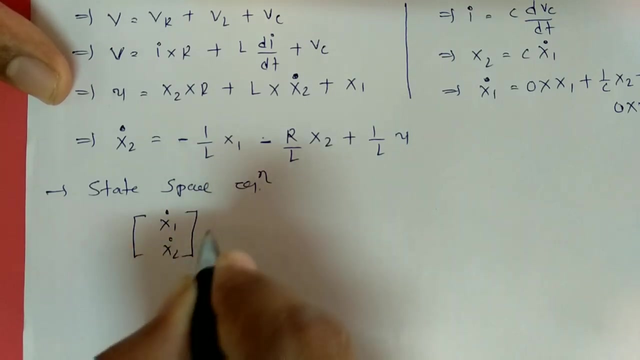 That is how I can write this. Now, by using this two equation, I can be able to write this state space modeling equation, which is what of x bar equation? So let us write this. So here state space equation that I can have by x1 bar, x2 bar and that too by x1 bar, that is, having this two coefficient, 0 and 1 by c. 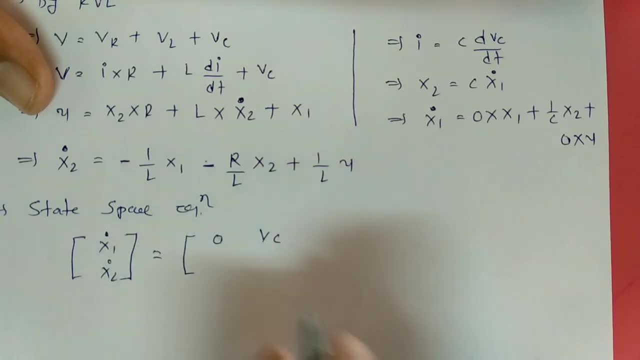 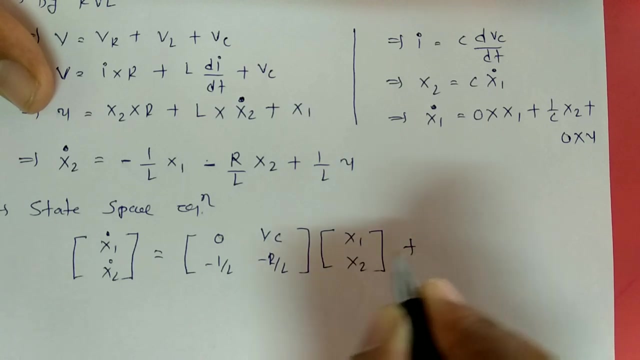 So let us write it: 0, 1 by c and x2 bar is having this two coefficient minus 1 by l and minus r by l, And that is getting multiplied with matrix. x1 and x2 plus u is having this coefficient for x1 bar. 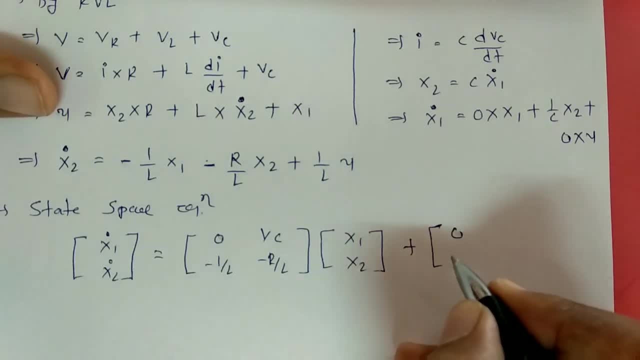 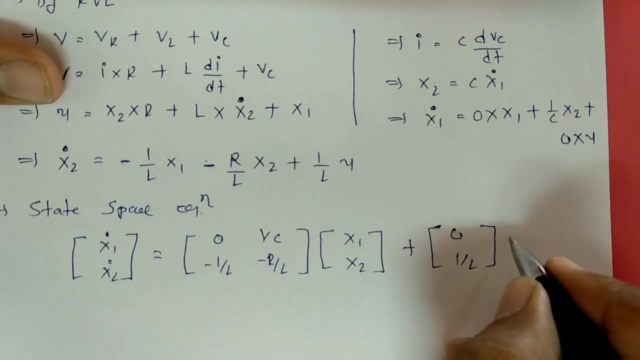 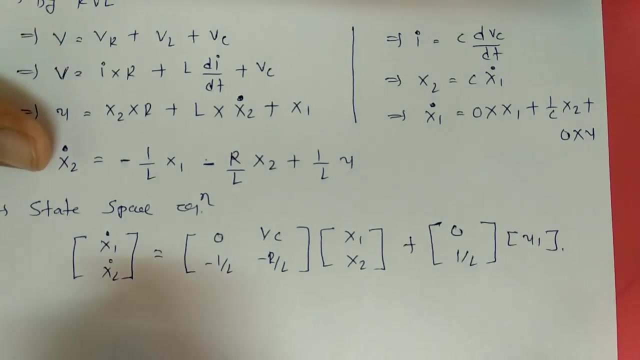 So it will be 0 over here and here it will be for u1.. Here it will be: x2 bar is having 1 by l, So that has to be 1 by l over here and into u1.. So that is how we have this equation. And now here one can say: this is what differential form of x1 bar. 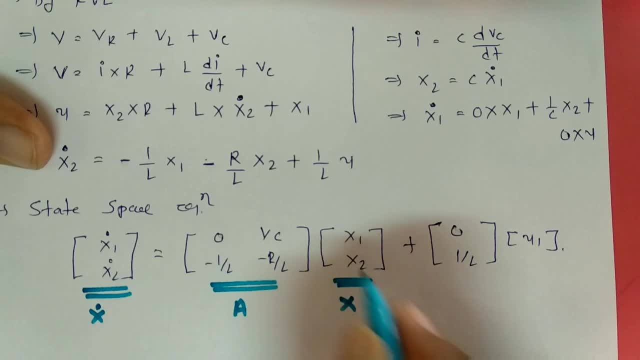 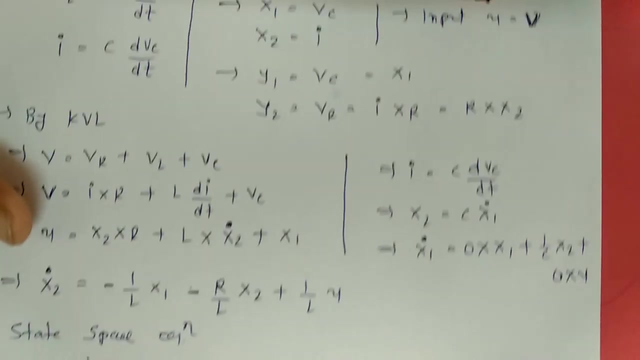 This is matrix A, This is matrix X. which is what state space matrix? This is matrix B and this is matrix U. So that is how one can have state space equation for electrical system. Now to have output equation. we have already derived this over here. 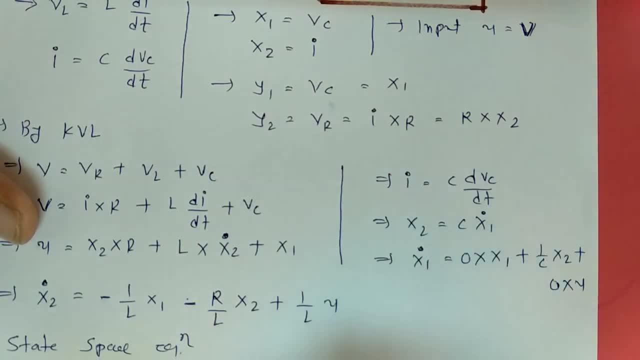 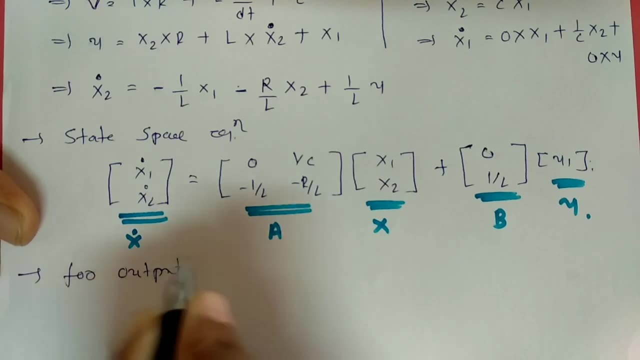 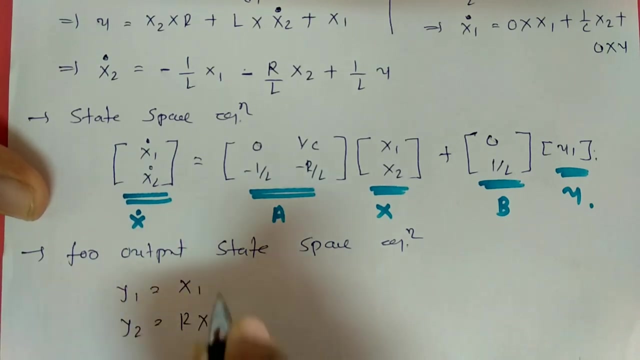 y1 is equals to x1 bar, x2 bar. So that is how we have this equation y1 is equals to x1 and y2 is equals to r2- x2.. Let us write it over here. So for output state space, equation y1 is equals to x1 and y2, that is actually rx2.. Let us rewrite this. 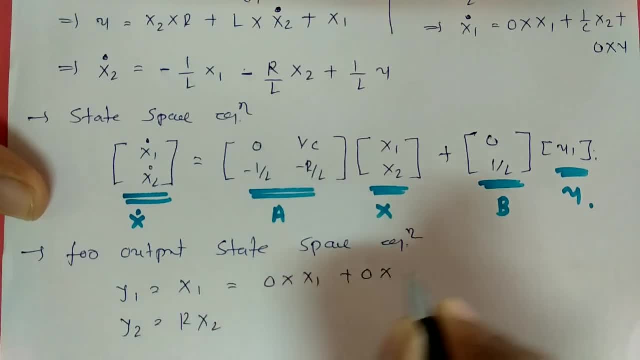 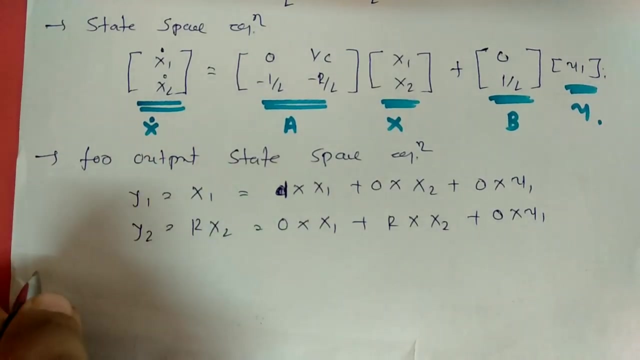 So 0 into x1 plus 0 into sorry, 1 into x1 plus 0 into x2 plus 0 into u1, and this will be 0 into x1 plus r into x2 plus 0 into u1.. Now to have matrix form in terms of output, that will be in terms of y1 and y2, that is equals to. this matrix will be: 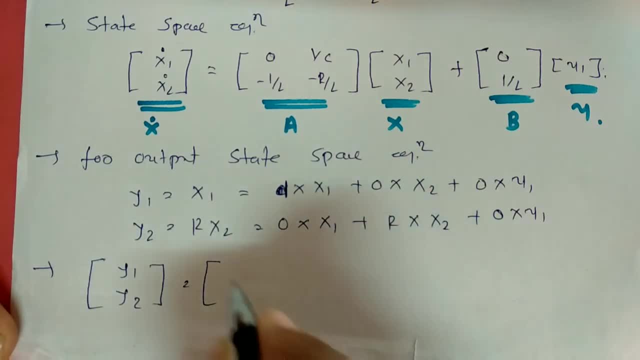 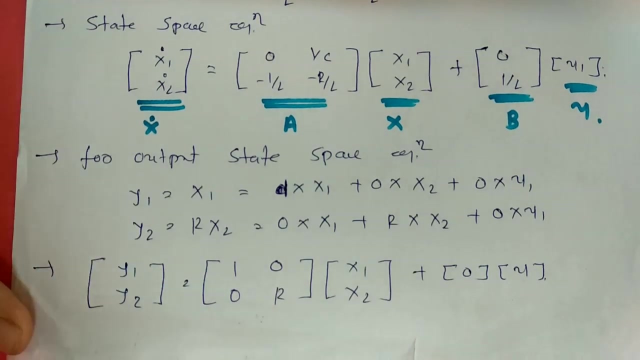 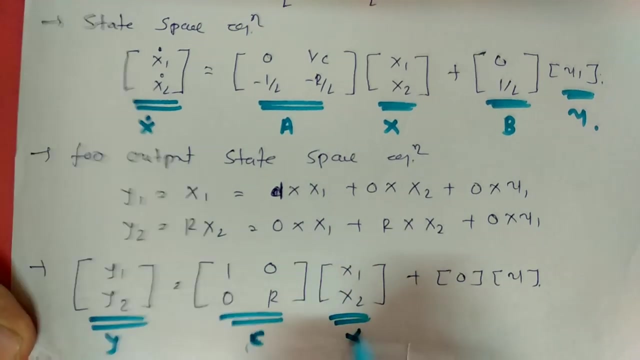 1 0 0 r, So 1 0 0 r into x1, x2 plus, this matrix is 0 and this is what u, So that is how one can have this and this is what our output. matrix y: This is matrix C. This is matrix X. state space matrix: This is matrix D, which is what having relevance with output.